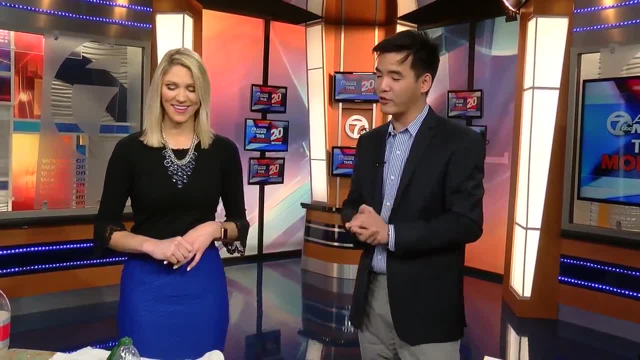 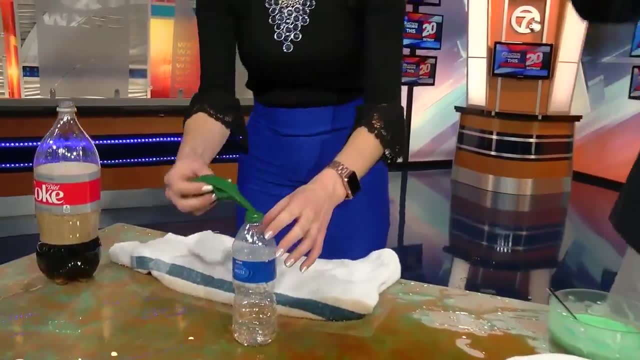 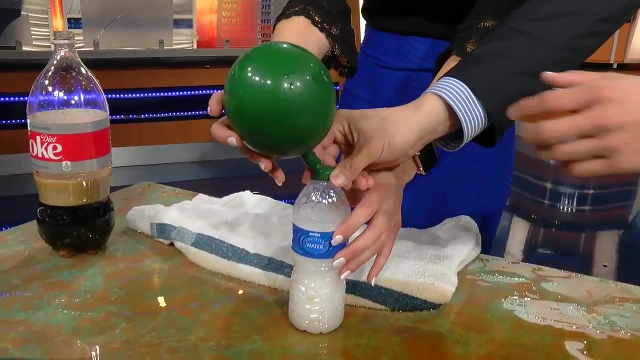 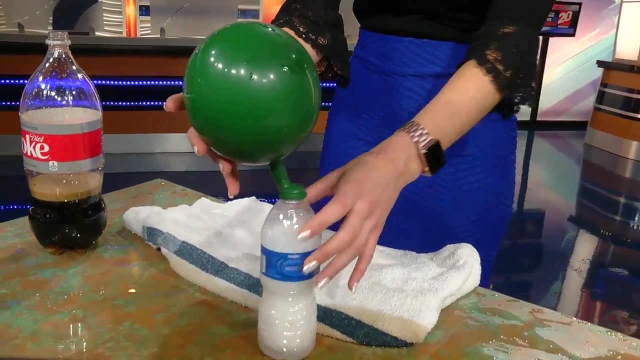 Through photosynthesis, So a lot of STEM and science terms too. that goes along with this. I love it. Very cool, The. I will let you basically just kind of dump the dump, Yeah, lift that up and just let it all kind of go in there and start to fill up. Look at that, The end. That is very cool And it'll get bigger as you. and another thing that you can work with your kids on is you can kind of balance and play around with the mixture of baking soda and vinegar and it'll blow up the balloon. 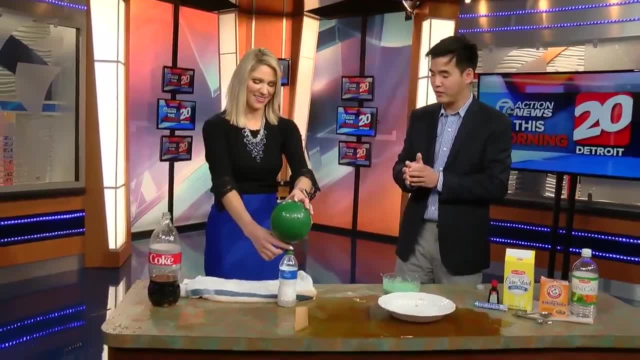 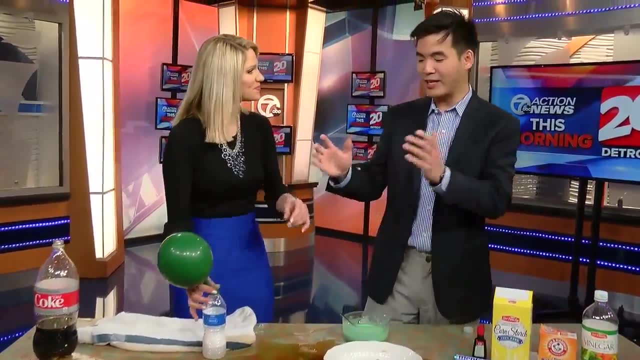 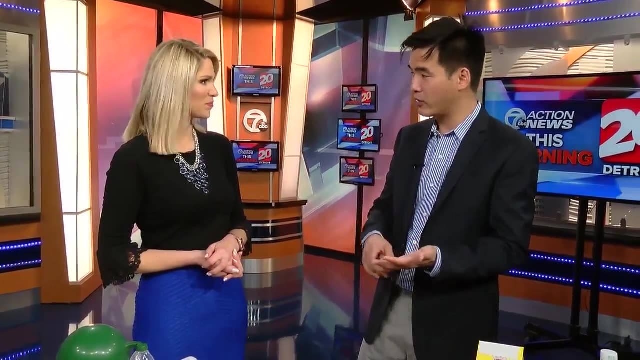 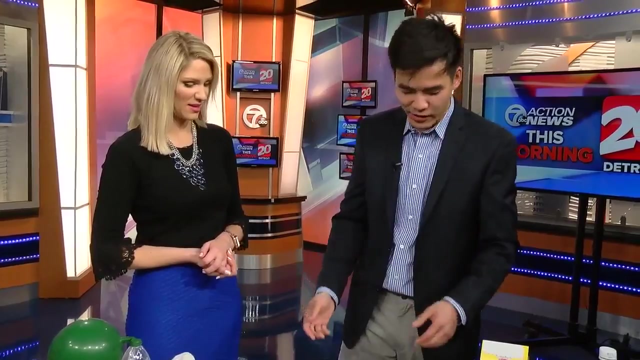 Based upon the varying mixtures that you do. I love this. This is super cool. And this is another cool one you brought here, Yes, So on the topic of gas, So we also know there's. the kids will learn. there's different states of matter, So there's, there's, obviously, solids, there's liquids, there's gases and there's plasma. So this is a pretty cool one where you, where you mix cornstarch with water, You throw in a little bit of dye, whatever you want Fun, Make it fun. Maybe some Diet Coke. 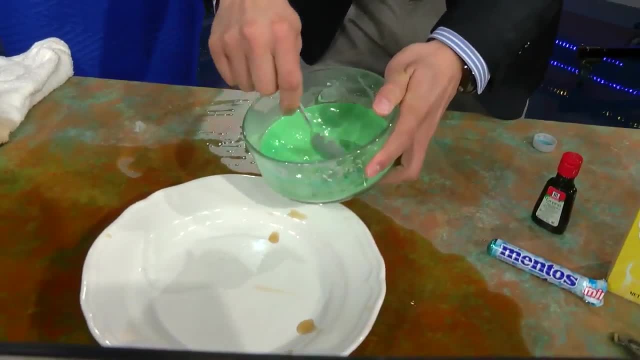 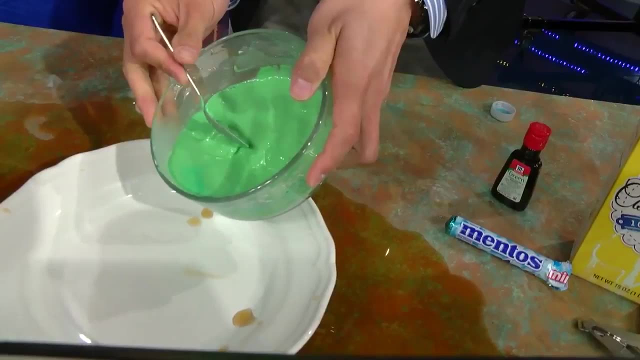 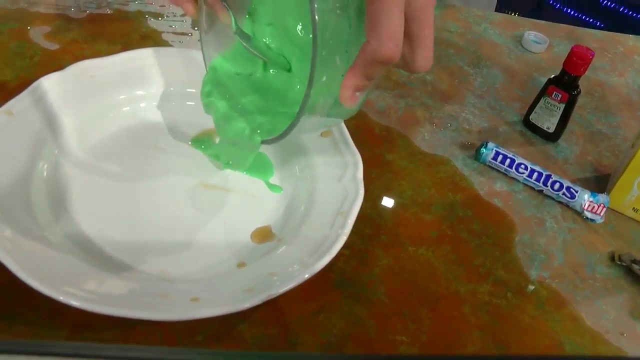 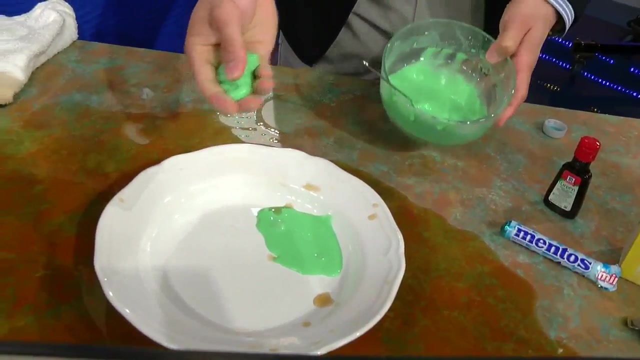 There's some Diet Coke in there too, And you basically, when you mix it up, it's going to be a little bit clumpy, But, as you can see, it's really cool because you can talk to your kids about, hey, so see how it's kind of formless, like like a liquid, You can pour it And once you let it all pour out, But then the cool thing about it is when you actually pick it up it feels like a solid. So it's going from a liquid to a solid And you can talk about the different states of matter in that way. So my nephews would love that. They love anything gross. 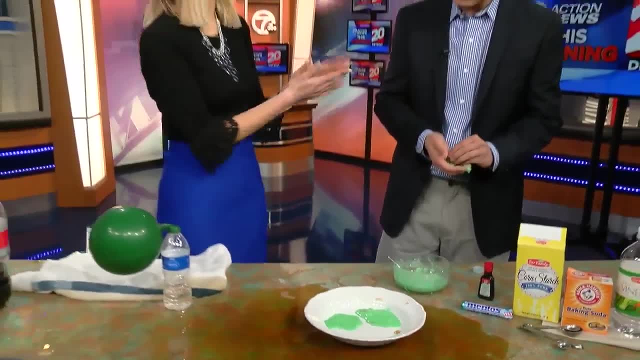 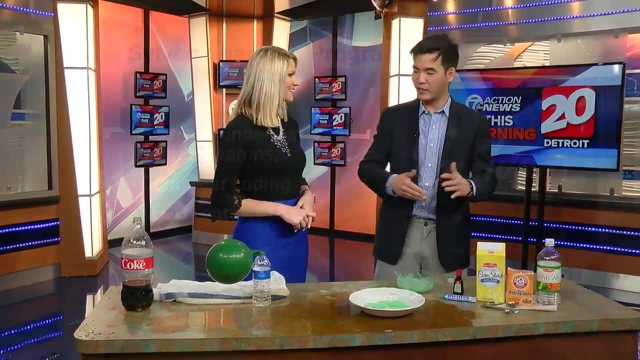 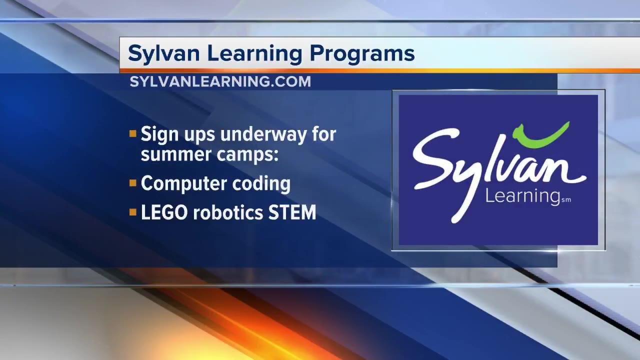 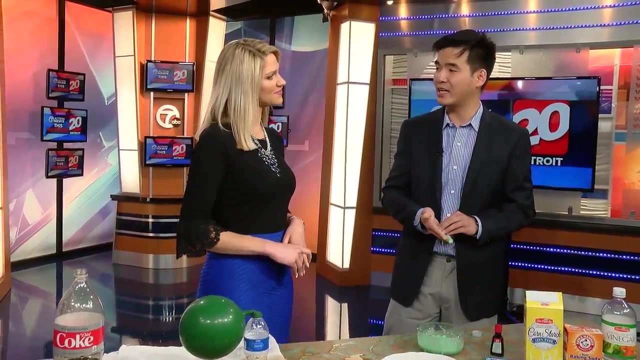 Right, Oh yeah, That is really cool. How fantastic. You guys have some summer camps coming up. Yes, we have a lot of camps, So we have this is called our maker space portion, where kids will basically go out. We'll do all sorts of fun and sometimes disgusting activities that the kids will love, And then we also have computer coding, Lego, robotics classes, as well as our award winning reading, math and writing, SAT and ACT classes too. All right, So the learning center dot com, Absolutely All right. Thanks so much for joining us. That was a lot of fun. I appreciate it.